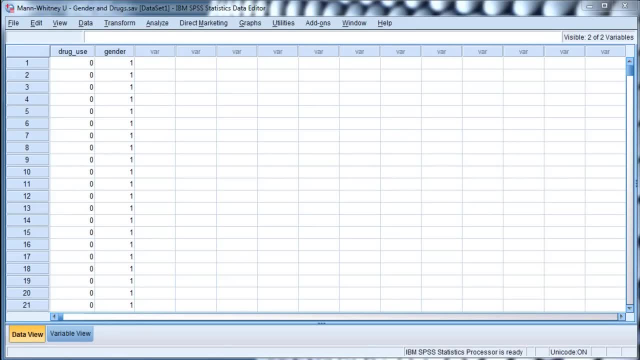 on an ordinal scale that is not sufficiently informative to allow an independent sample t-test to be performed In this case, which is fictional data. what I have are two variables: the dependent variable, which is drug use, and let's just say this is the number of times that 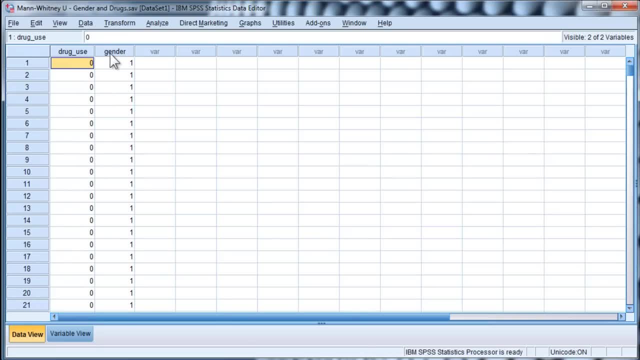 young adults report having used drugs before, and gender is the independent variable and that's coded 1-2 for males and females, and the hypothesis here is that the measures of central location in the context of Mann-Whitney U, the mean ranks, are unequal. Now I'll just show you briefly that. 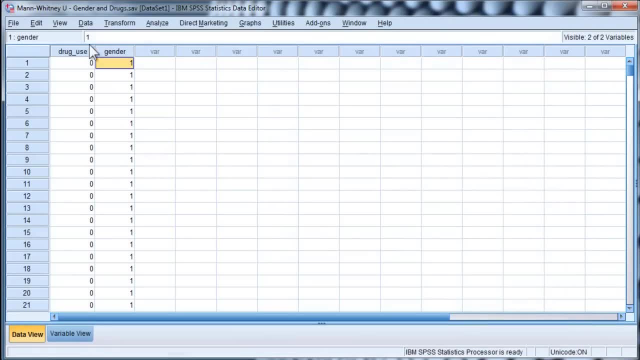 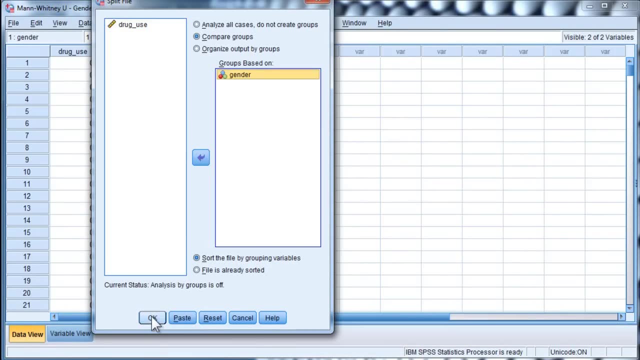 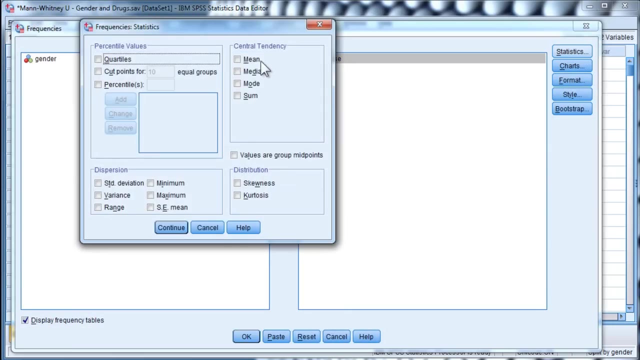 the data are quite substantially non-normally distributed and to do so I'm going to split the file and compare groups according to gender and look at the frequencies and just get some basic descriptive statistics: mean median skew, kurtosis and histograms. Now a lot of people will look at the distributions. 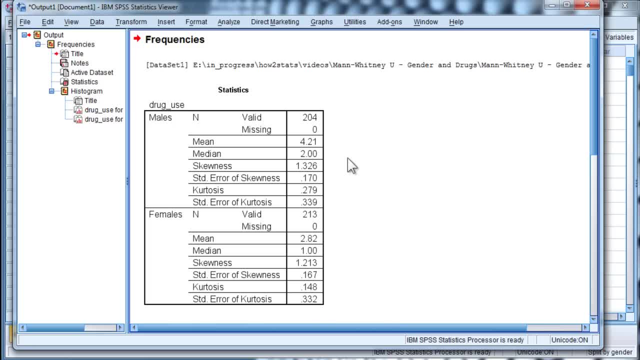 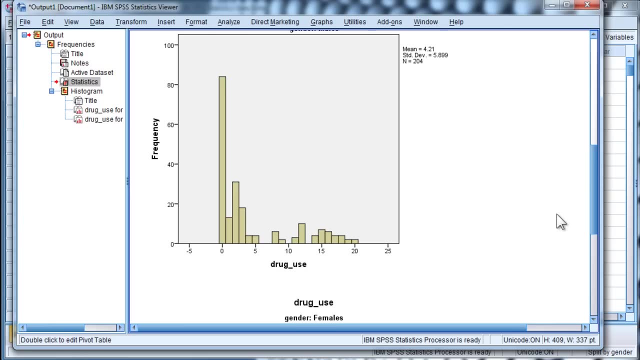 for the whole sample, when really you have to look at the individual groups separately, We can see that skew for males is 1.33 and females is 1.21, and if you look at the distributions, these are data that are arguably fairly substantially skewed. 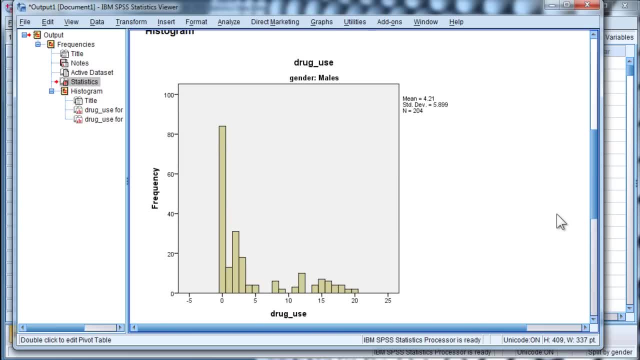 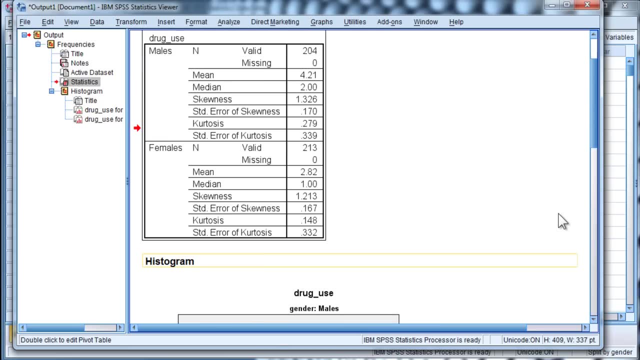 Now whether an independent sample t-test would accommodate this or not is a separate question. Let's just say that it can't, that the data are sufficiently non-normally distributed that you'd want to do a non-parametric statistic like Mann-Whitney U. 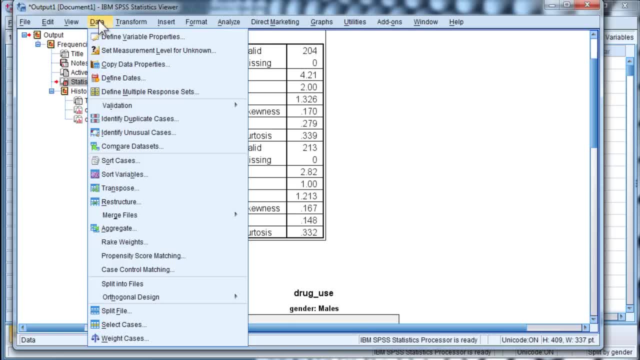 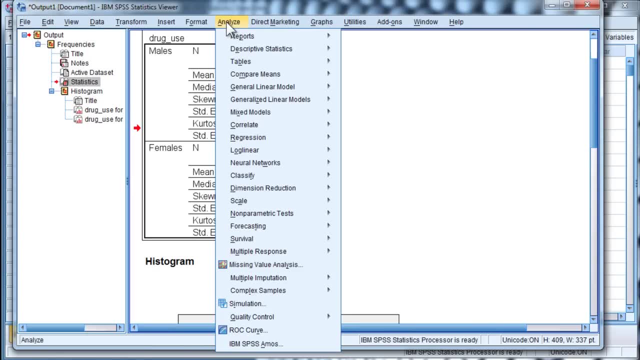 Now to conduct the Mann-Whitney U, I'm going to have to unsplit my file, analyze all cases and go into Analyze and Compare Means, or I should say Non-Parametric Statistics, Legacy Dialogues and two independent samples. 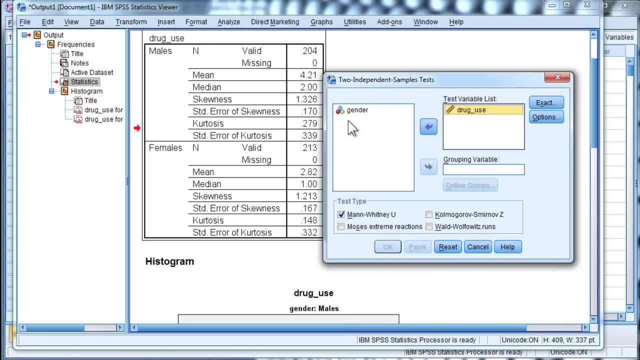 And I've got Drug Use as my test variable list and Gender as the grouping variable. I'm going to define the groups as 1 and 2, so you have to do this because you might actually have a group with four different. you might have an independent variable with four levels. 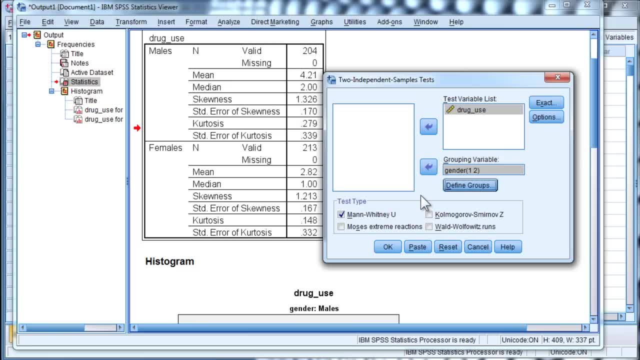 and you have to tell SPSS which of the two groups that you actually want to compare. Now, the default is Mann-Whitney U, and that's the one that I'm going to use. So I'm going to use Mann-Whitney U. 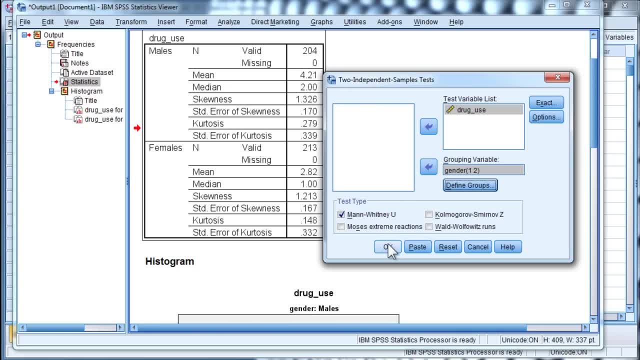 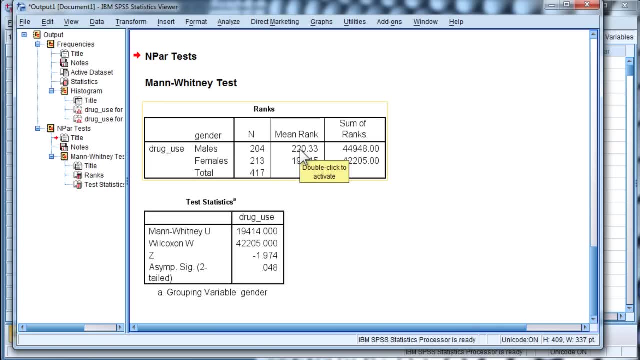 and you select the two independent sample tests and click OK And here we have the mean ranks. You don't get the descriptive statistics, like the mean of drug use. You only get that if you look at the descriptive statistics. So for males it was 4.2,. 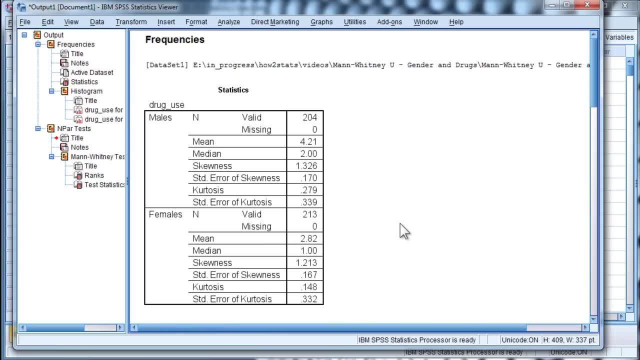 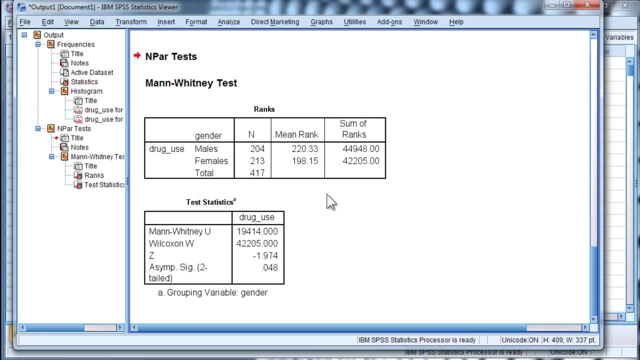 and for females 2.8, so at least numerically, males are scoring higher than females. We don't know if it's statistically significant and because it's non-normally distributed, we had to use a non-parametric approach. 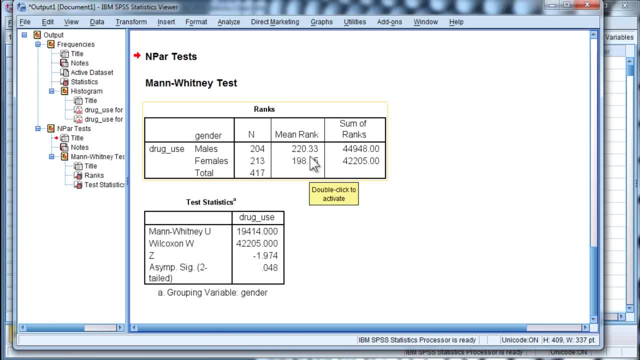 which is the mean ranks in this case, and the males have a mean rank of 220, and the females have a mean rank of 198.. Now is that numerical difference statistically significant? Well, we can look at the Z statistic here. 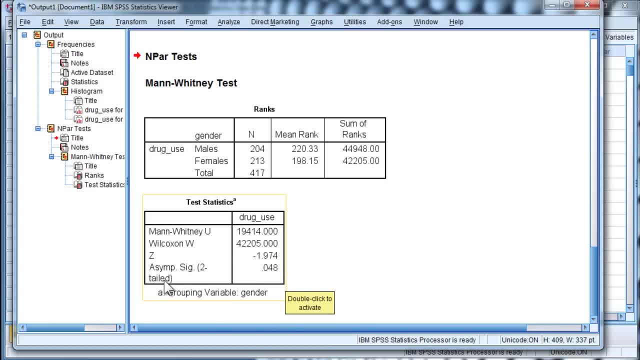 which is negative 1.97, and the P value is equal to 0.048.. Now, because this P value is less than 0.05, we would reject the null hypothesis of equal mean ranks. So in this case, 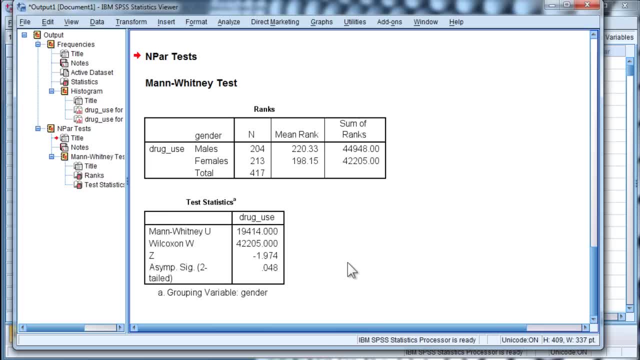 we could assert that males have a higher level of reporting drug use than females based on this sample. Now a second question that you'd want to ask here is the effect size, and a lot of people don't know this, but you can calculate an effect size from a Mann-Whitney use statistic. 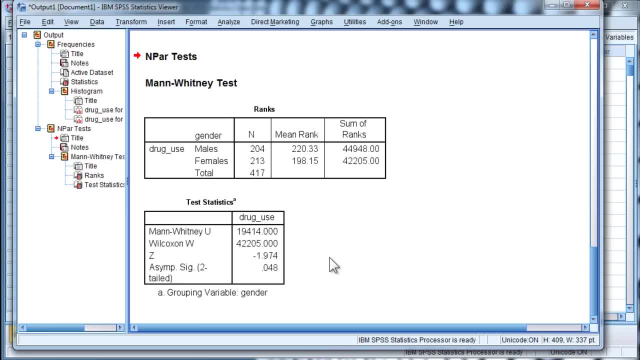 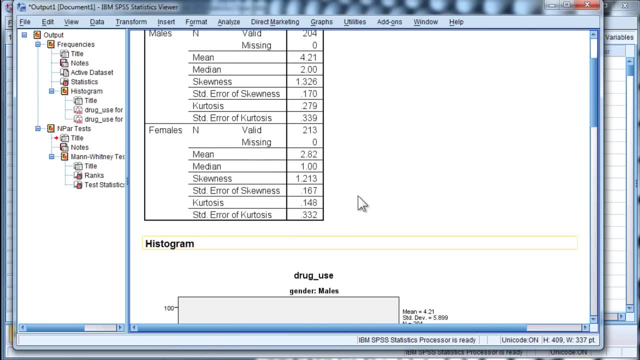 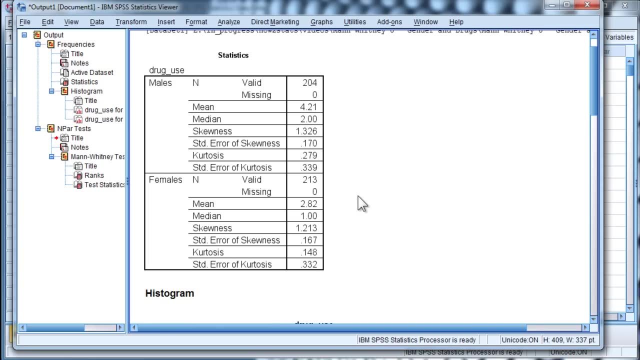 I'm going to do that in a separate video, And I'll also point out that non-parametric statistics like the Mann-Whitney use actually do have assumptions. Now, they might not assume normally distributed data, but they do assume that the data are non-normal. 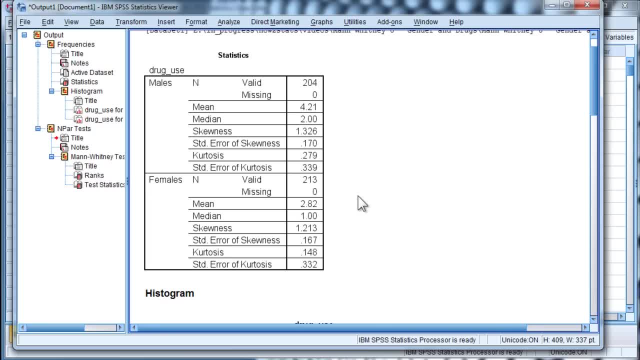 in the same way for all of the groups included in the analysis. Now, in this case, we have skew of 1.3 and 1.2, and I could have looked at the standard deviations as well, So I'm just going to briefly show you. 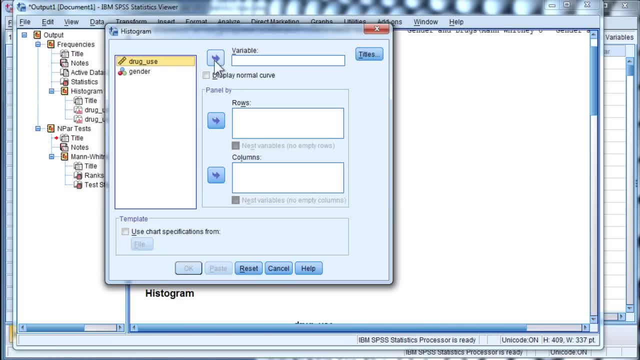 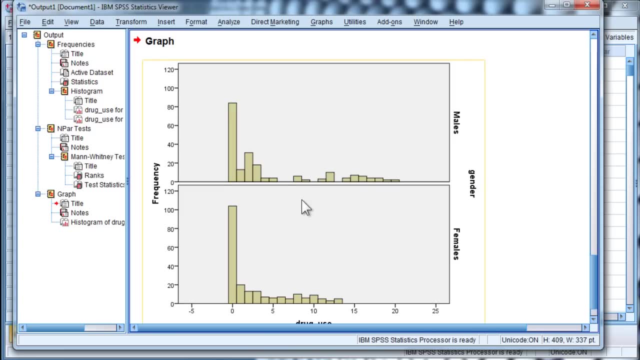 a histogram that lets you look at the two groups a little more closely or more comparably with this histogram here, And you can see that the males really do actually have a different distribution than the females. They're both positively skewed, but the males are much more so than the females. 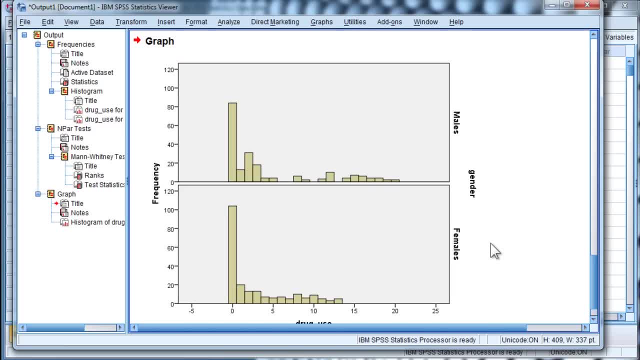 This is concerning. Like. a lot of people do not know this, so you can get away with doing the analysis as I've just reported it, But I would be concerned that these data are too differentially non-normally distributed for males and females. 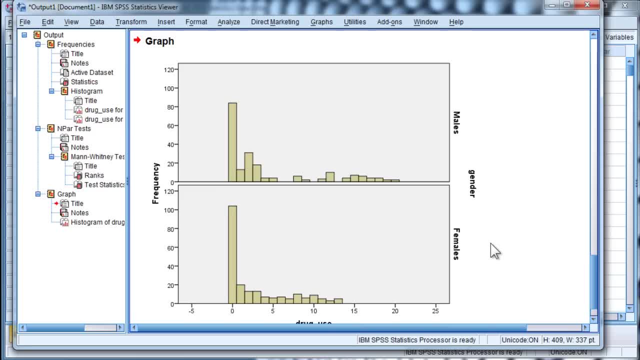 And I'll show you in another video how to test the assumption of equal distributions for males and females, to satisfy the assumption of the Mann-Whitney use statistic. So I'm going to follow up with two videos, one for effect size and the other one for testing the assumption. 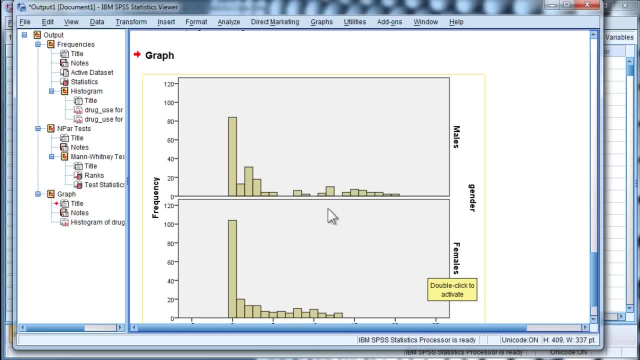 of similar distributions between your groups. Thanks for watching. 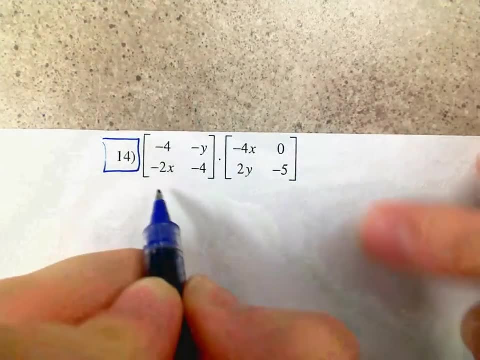 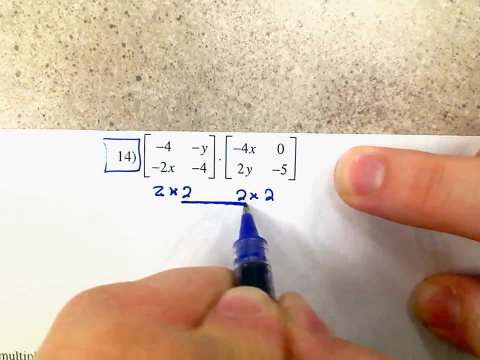 Okay, number 14, I've got a 2x2 matrix here and a 2x2 matrix here. If the inside numbers are the same, I can multiply them, because the columns of the first one will be equal to the rows of the second. 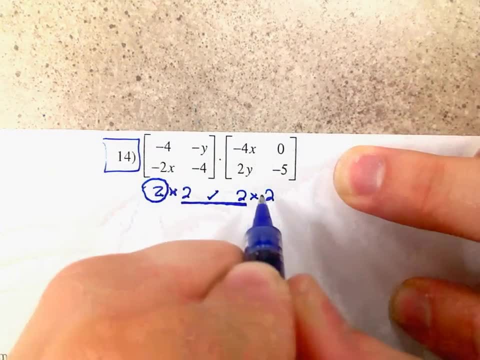 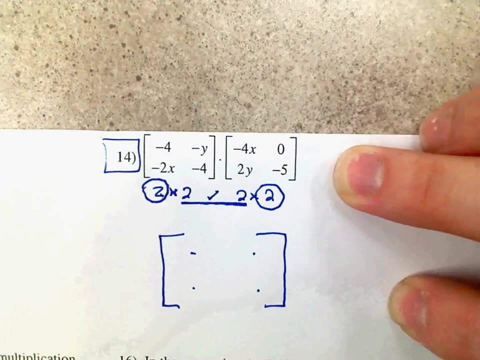 So what I'm looking for now is: what type of matrix will I have? Well, the outside numbers tell you that it's a 2x2.. So I'll have exactly four answers here. So the first one will be the first row and the first column. 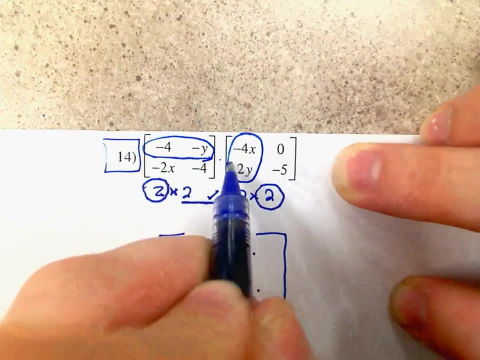 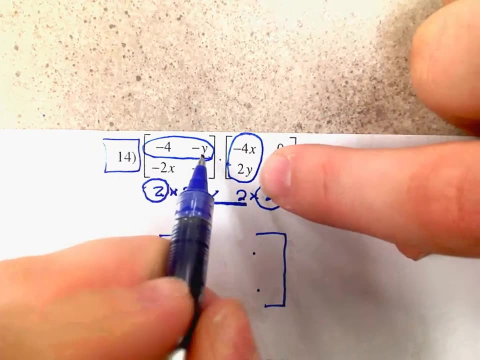 So grab your first row times, your first column. Now I've got negative 4 times negative 4x- that would be positive 16x. And negative y times 2y- that would be negative 2y. squared. Normally you add these together. 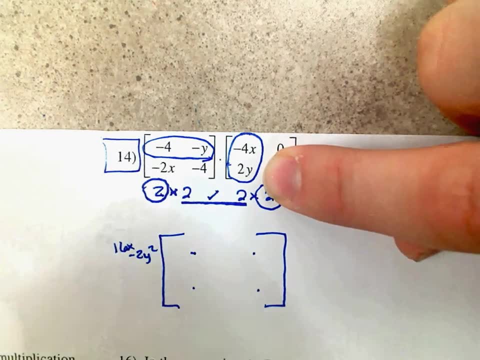 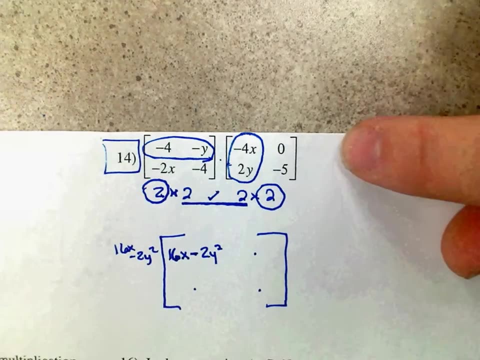 You can't add together an x variable with a y variable, so we're going to leave them the way they are: 16x minus 2y squared. Okay, then we're going to jump here. first row, second column, Negative 4x.